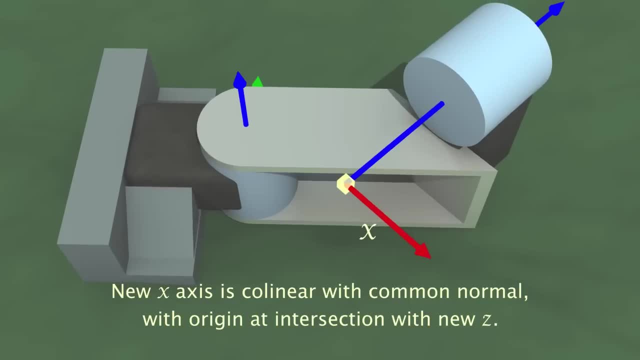 The new x-axis will point away from the previous joint. The y-axis will point away from the previous joint. The z-axis points along the common normal and has its origin at the intersection with the new z-axis. Notice: the origin is not within the physical actuator because 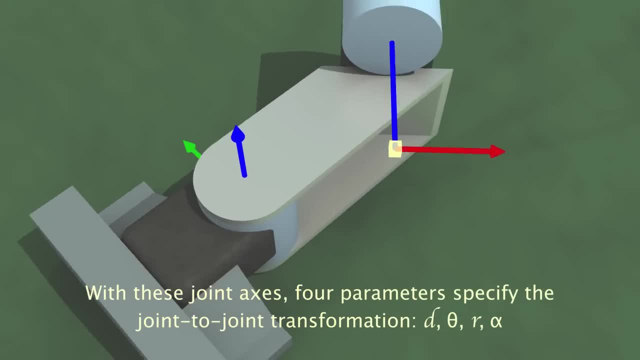 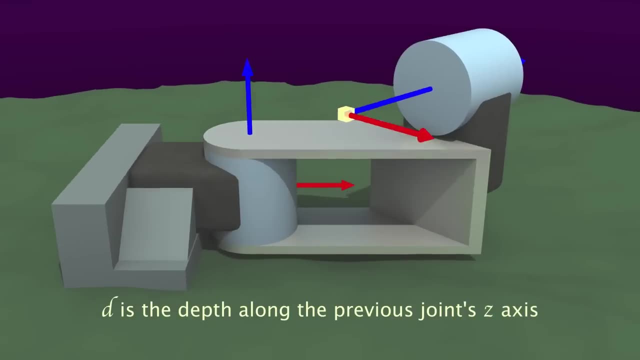 the dh-parameters are only concerned with the motion of the links, not the physical placement of components. Using this protocol, for laying out the reference frames, only four parameters are needed. The first of these, d, is the depth along the previous joint's z-axis from the origin. 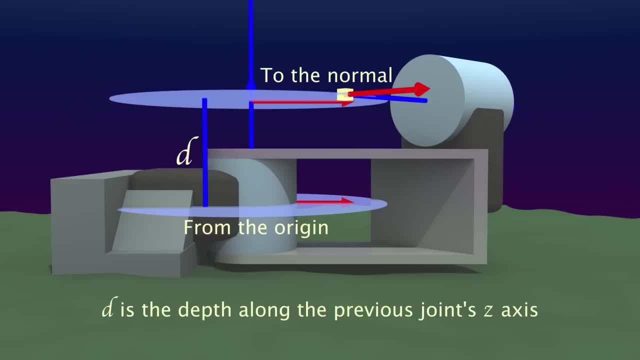 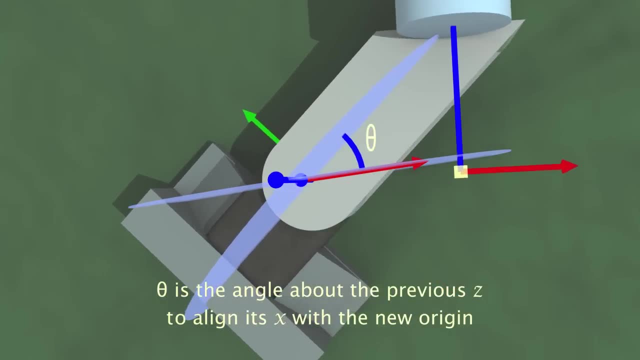 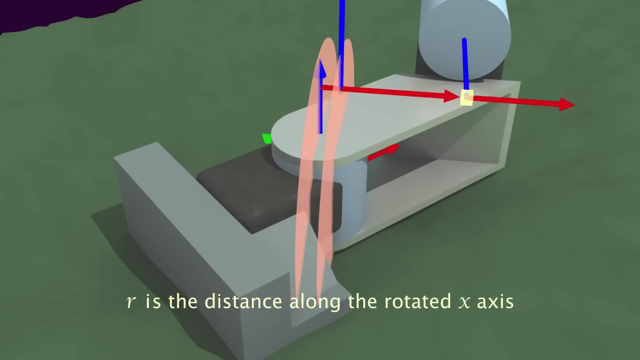 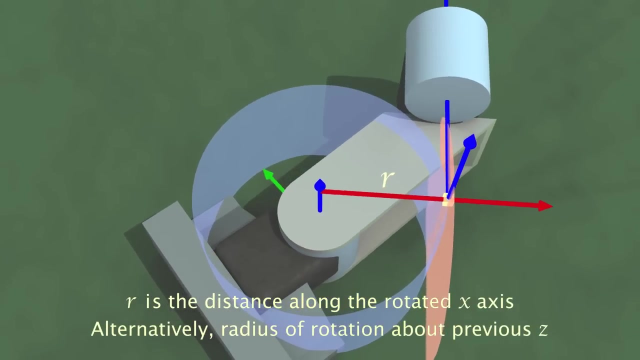 to the common normal. Theta rotates about the previous z-axis to align the x-axes. R is the length of the common normal itself. Most texts call this parameter a, which is unfortunately easy to confuse with alpha. Instead, calling it r is a useful monomic. 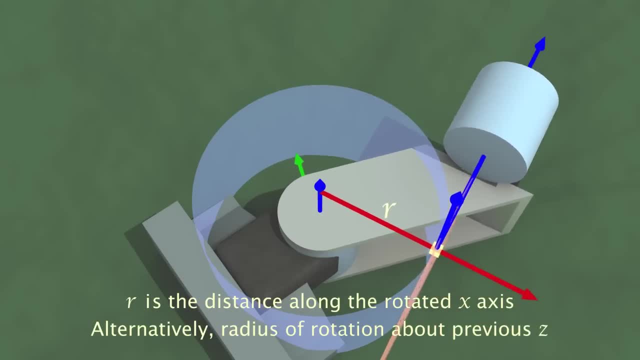 as this is also the radius of revolution for the new origin about the previous z. Finally, the radius of the new z-axis gets the same length as the previous z-axis. We will also find the radius of previous z-axis, which is the radius of the new z-axis, which 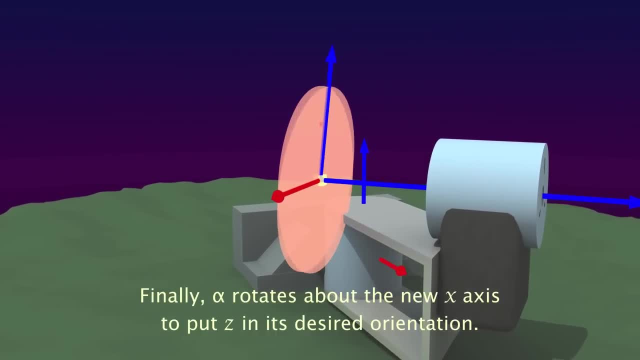 is also the radius of the previous z-axis. Finally, if we calculate the new z-axis at the intersection, we find that the z-axis is Finally alpha rotates about the new x-axis to bring z into alignment with the axis of joint motion. 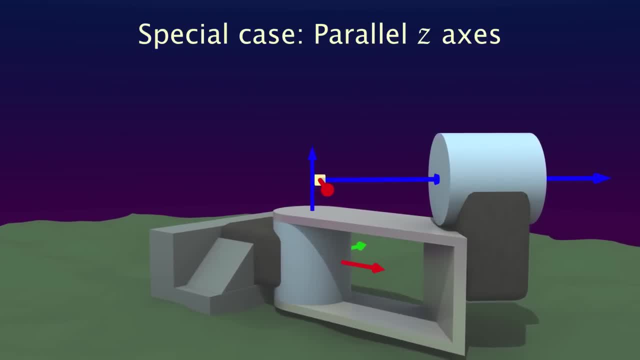 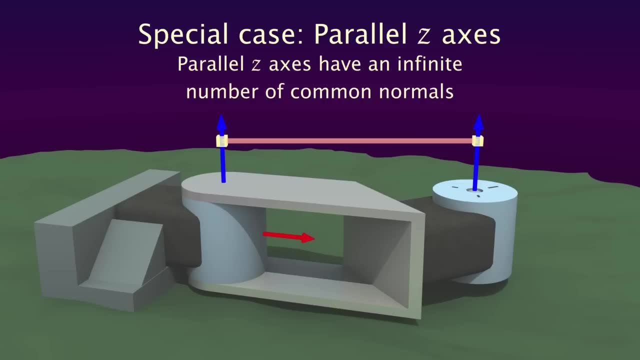 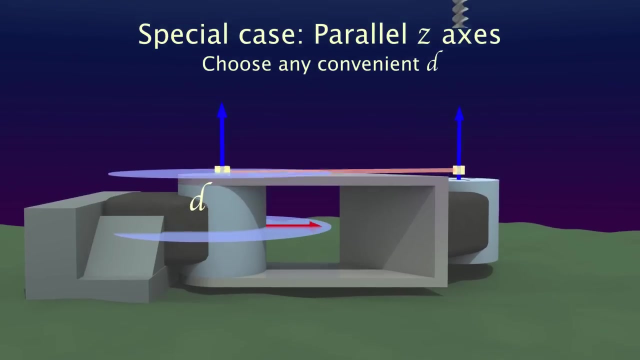 Now there is one special case: when the z-axes are parallel, Because parallel lines have an infinite number of common normals, you can choose any d-value you like in order to place the new origin at a convenient location, such as the center of a link or the tip of an end-effector. 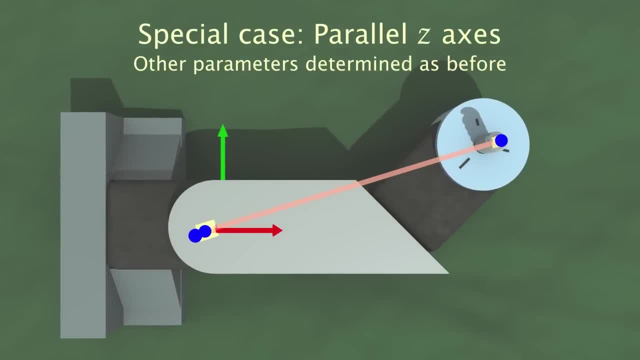 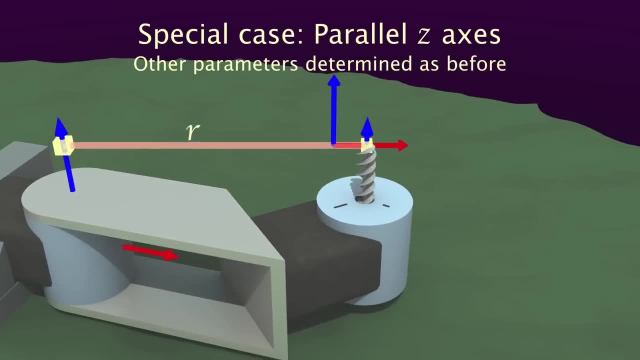 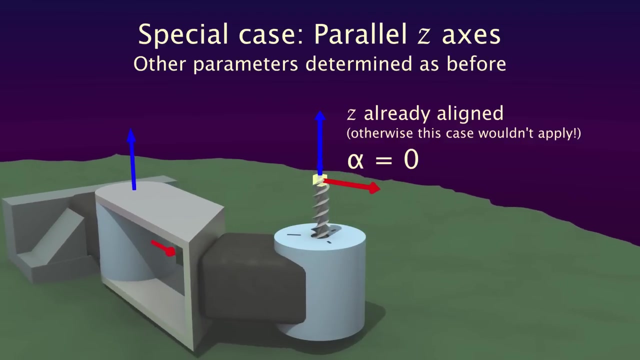 The other parameters are the same as before. Theta rotates about z to align the x-axis with the normal, and r translates out along the normal to reach the new origin. Alpha is already known to be zero in this case, since the z-axes must be parallel for 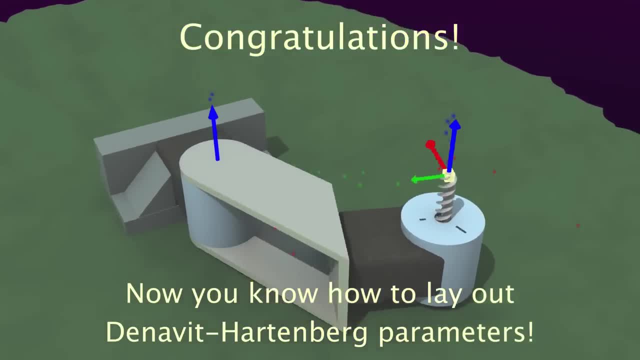 this to apply. thus, no rotation is needed. Congratulations, That's all there is to it. Thanks for watching.